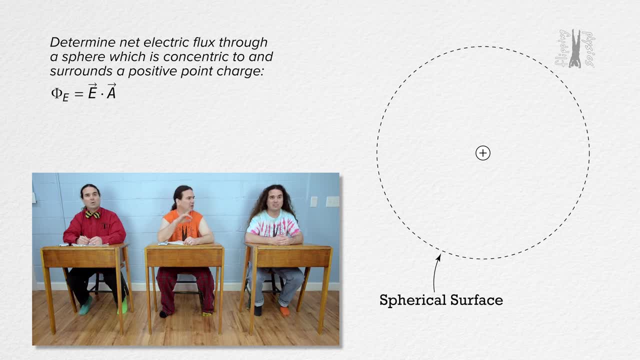 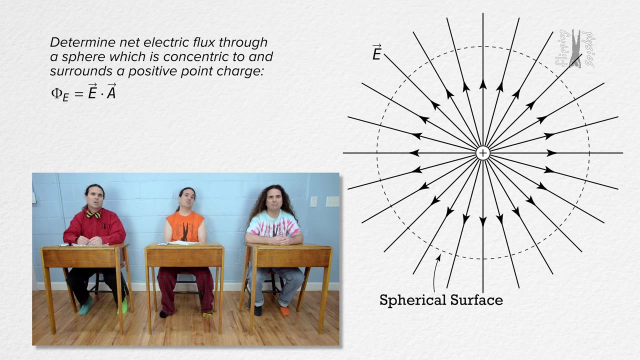 so let's use that. We know the electric field is. You can't use that equation, Why not? That is the equation for electric flux. when the electric field is uniform, The electric field caused by a point charge is not uniform. The electric field decreases as you get farther. 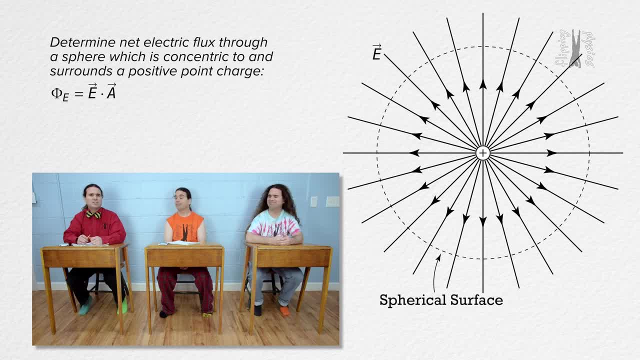 from the point charge. Yeah, We need to identify infinitesimally small areas of the surface, which are dA, and the infinitesimally small flux is d phi, created by the electric field passing through dA. Actually, rather than using fluxes for the plural. 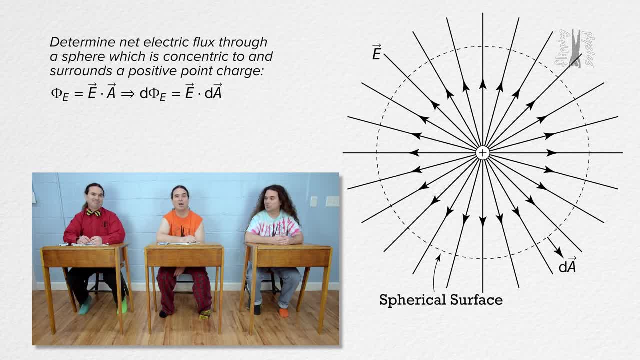 flux, I'm going to say electric flux values. Of course you are Yes. Take the integral of both sides and we get an equation for electric flux which does not need the electric field to be constant. Electric flux equals the integral of the dot product of 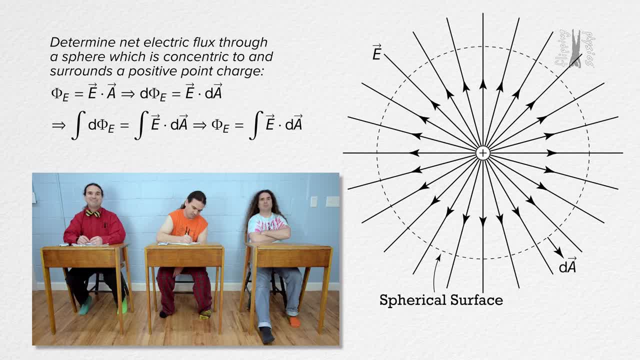 electric field and dA. Okay, let's use that equation. However, let's use e, dA, cosine theta instead of the dot product. The angle between the electric field and dA is, for every area of dA, equal to zero. That is because the electric field is always. 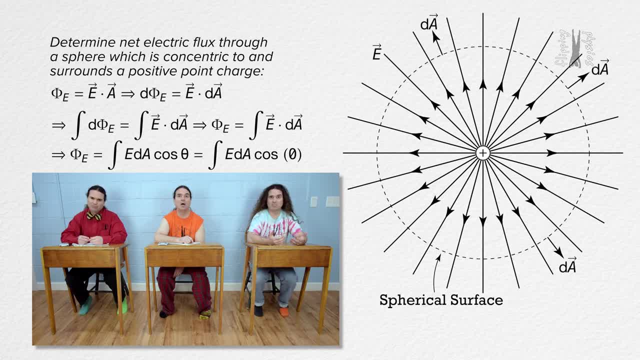 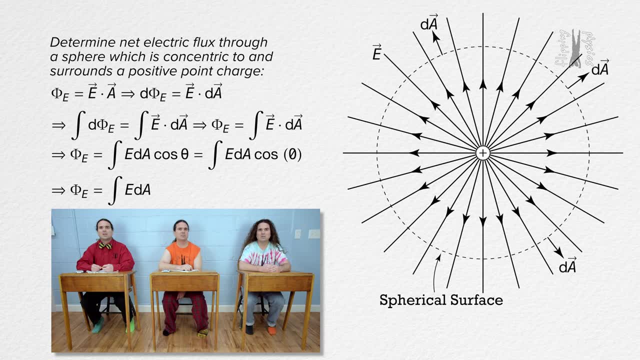 outward and dA is always outward. They are both in the same direction. The cosine of zero is one. Actually, the electric field has the same magnitude as it passes through every infinitesimally small area of dA on the concentric-spherical surface, through which. 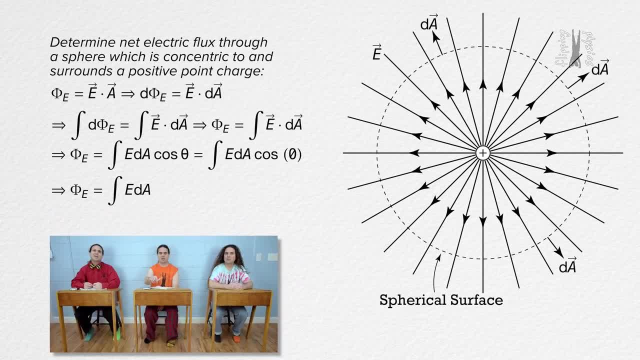 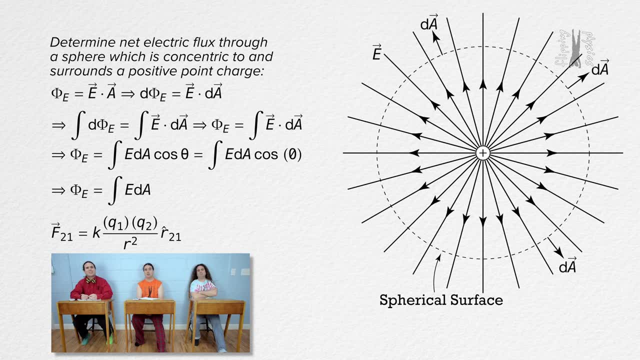 we are finding the flux. It does. Yeah, Coulomb's law gives the electrostatic force as the Coulomb constant times, charge 1 times charge 2, all divided by the square of the distance between centers of charge all times, unit vector r. 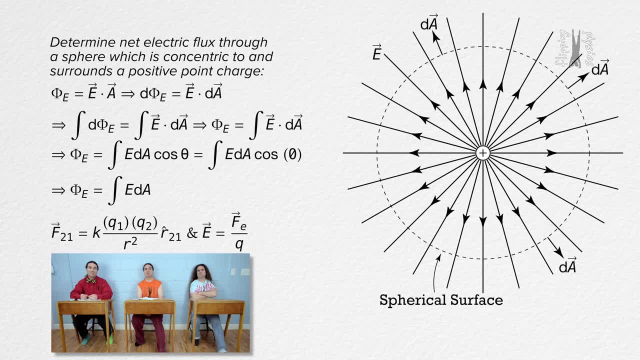 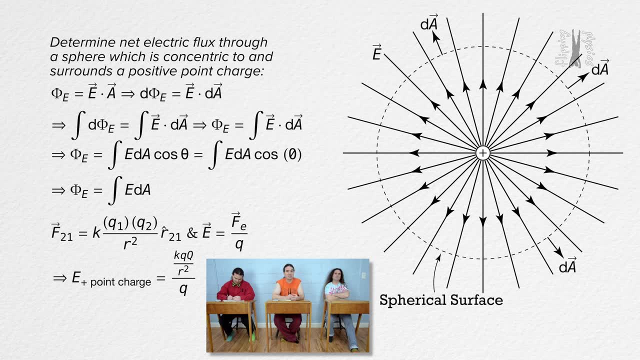 The electric field equals the electrostatic force divided by the charge on the small positive test charge. That means the electric field around a positive point charge equals the Coulomb constant times, the test charge times, the point charge, all divided by the square of the distance between: 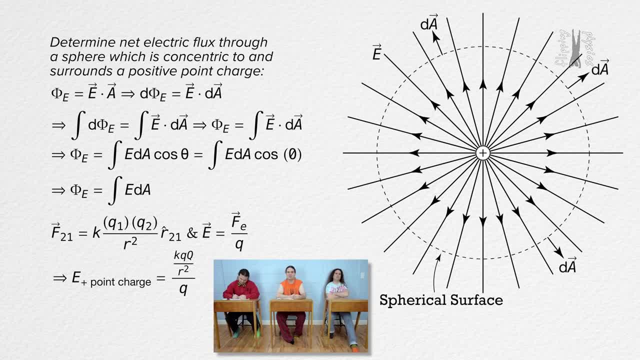 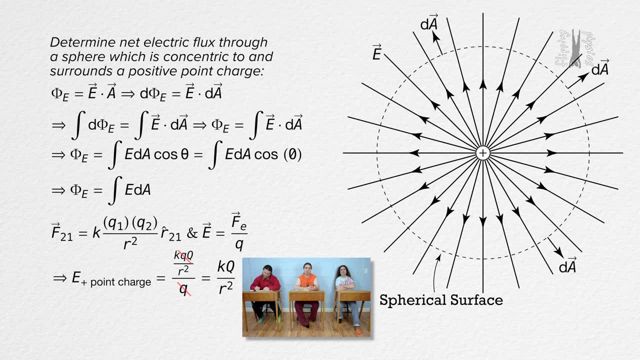 centers of charge. and all of that divided by the test charge. The charge of the test charge cancels out and the electric field around a point charge equals the Coulomb constant times the charge of the point charge, all divided by the square of the distance between the center of the 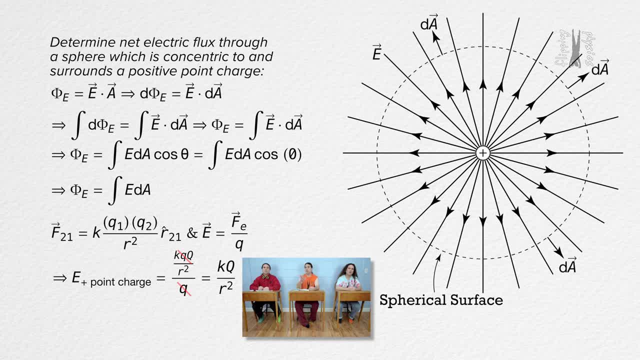 point charge and the location of the electric field, In other words the electric field which surrounds and is caused by a point charge, is constant at a constant radius. The concentric sphere has a constant radius, so the electric field which is moving is constant at a constant. 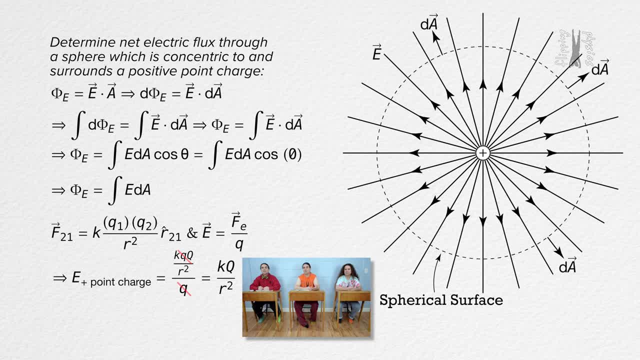 field there is constant, So we can take electric field out from under the integral. In other words, we could have just used the equation I started with, Maybe, but this is mathematically a more rigorous approach. Okay, The integral of dA is a: the area of the concentric spherical surface, The surface. 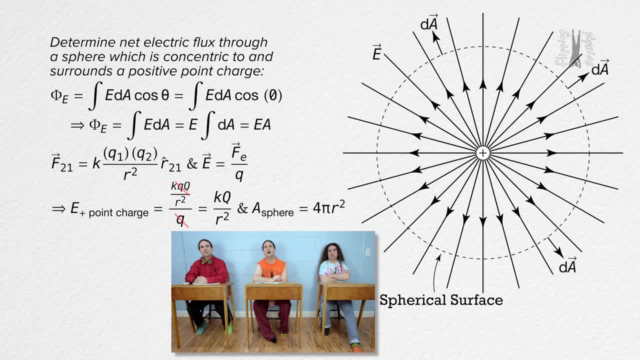 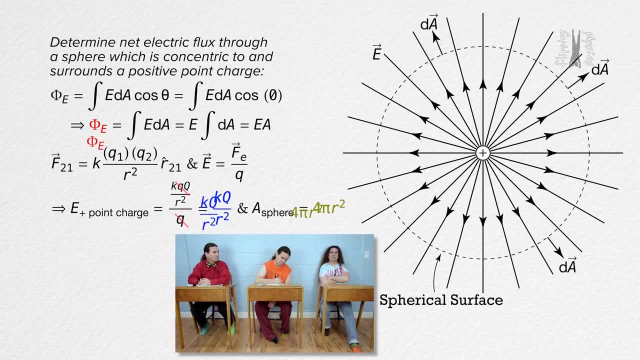 area of a sphere equals 4 pi r squared. We can substitute in the equation for the electric field which surrounds a point, charge and the equation for the surface area of a sphere into the electric flux equation The square of the distance from the center of the point. 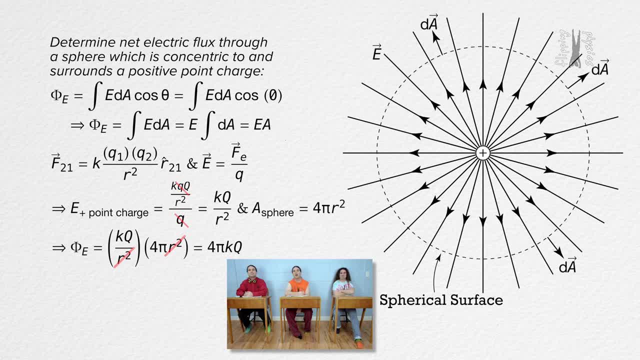 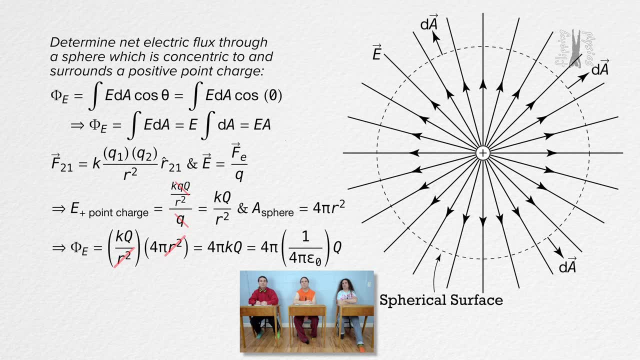 charge to the electric field cancels out, and that looks good to me. We also know the Coulomb constant equals the inverse of the quantity, 4 pi times the permittivity of free space. 4 pi cancels out and we get a more elegant answer. The electric flux, which 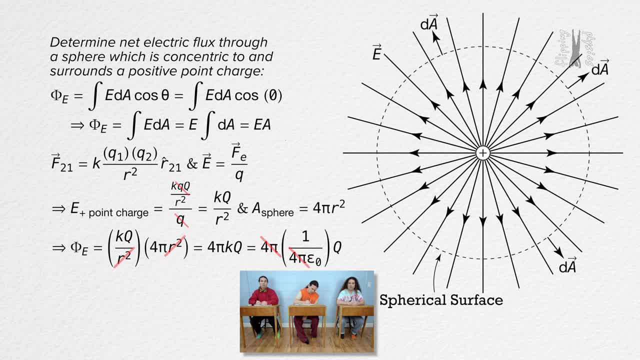 passes through a sphere which is concentric Concentric to a positive point charge equals the charge of the positive point charge divided by the permittivity of free space. Sure, A more elegant answer using a more mathematically rigorous approach. So the electric flux is independent of the radius of the concentric spherical surface. 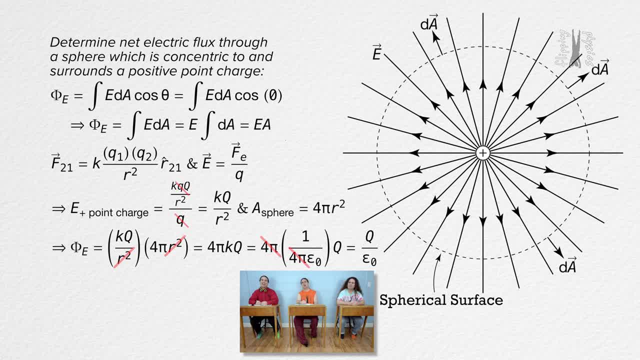 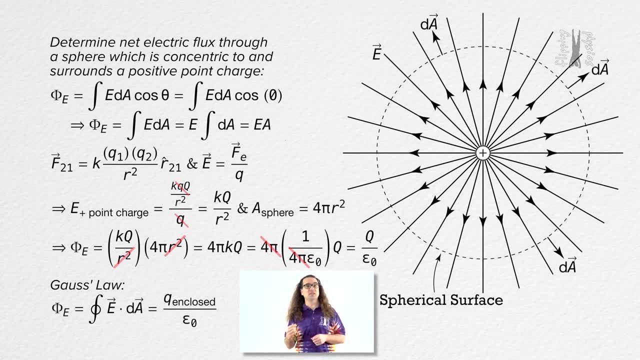 Cool That? that is weird. Yeah, Yep, And what we have just shown here is a demonstration of Gauss's law. Gauss's law says that a closed surface equals the closed surface integral of the dot product of electric field and area dA, which equals the charge enclosed in the Gaussian surface divided by: 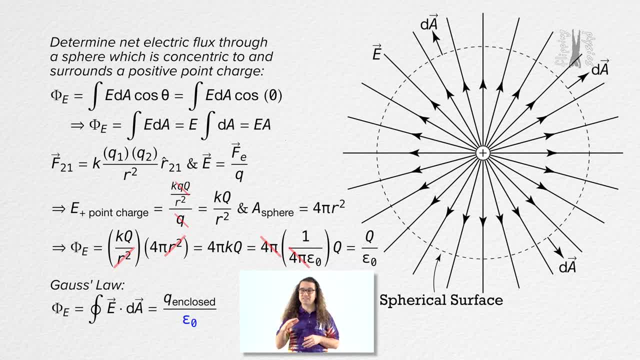 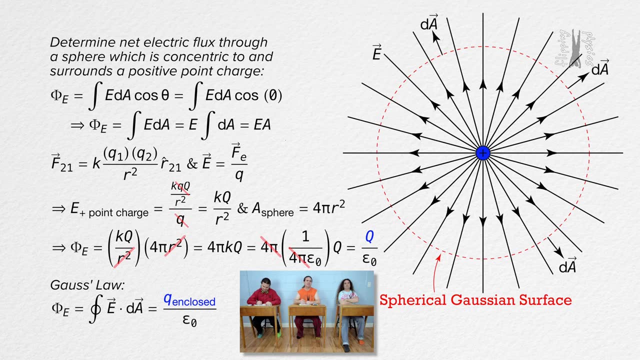 the permittivity of free space. In the example we just did, capital Q is the charge of the point charge and it is the charge enclosed inside an imaginary spherical surface, and the imaginary spherical surface is called a Gaussian surface. That circle in the integral sign is a point charge. 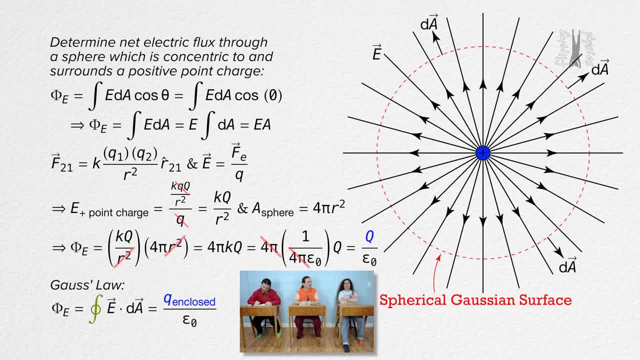 Yeah, That circle in the integral sign is confusing. It just means the integral is over a closed surface. It's called a closed surface integral. Okay, I guess that helps. Thanks, Sure More specifics about using Gauss's law. A Gaussian surface is a three-dimensional closed. 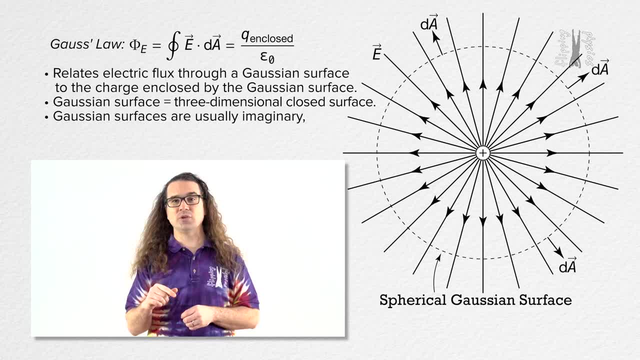 surface And realize, while the Gaussian surface we usually work with are imaginary, the Gaussian surface could actually be a real physical surface. Typically, we choose the shapes of our imaginary Gaussian surfaces based on the three-dimensional closed surface. Tack, I have no idea if that means I must overexaturate things. 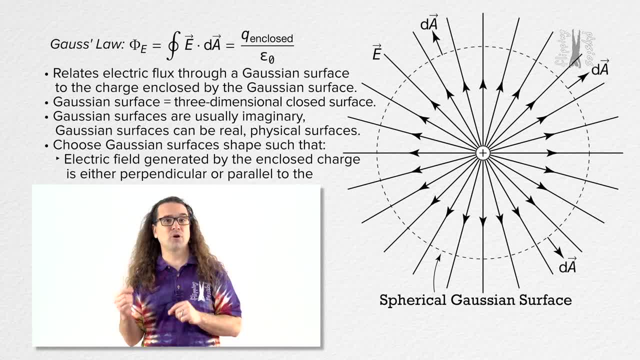 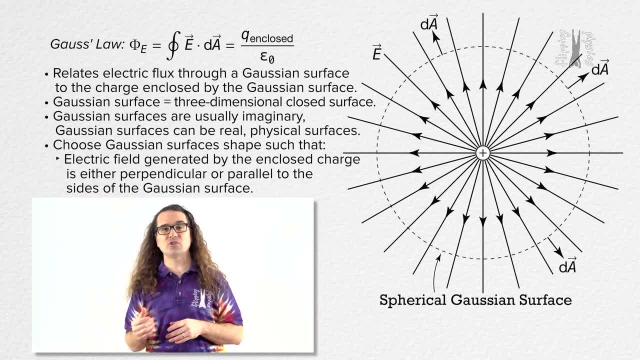 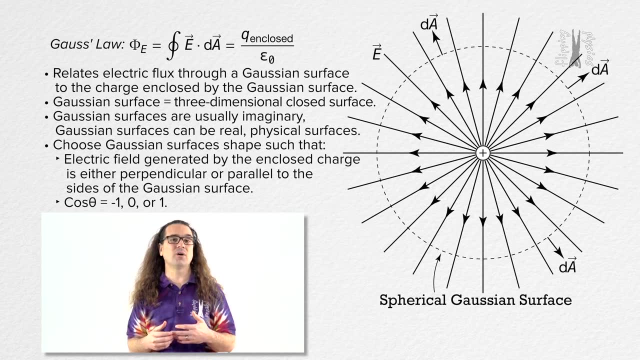 Yeah, that would be ло tort wall-plus-valueсп league, double p-brain. Sure, Just me mad. You're not going to let it work without me concentric with the point charge. The electric field and the area vector were always in the 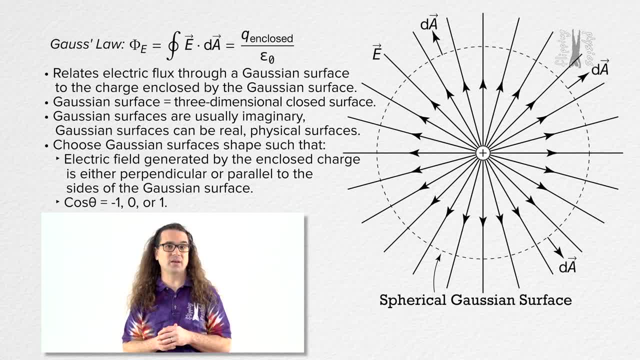 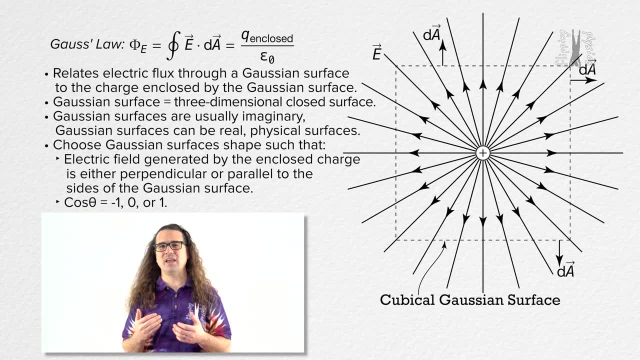 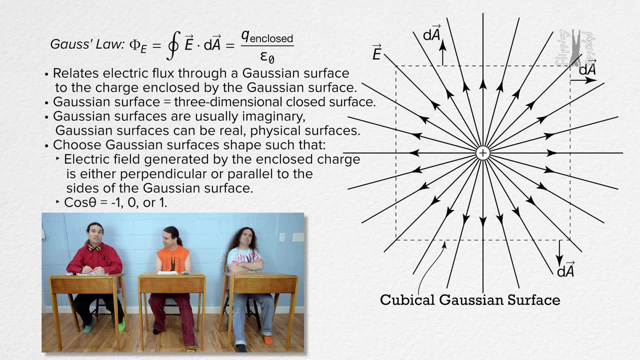 same direction, giving an angle of zero degrees in the dot product. If we had chosen a cube as our imaginary Gaussian surface, the angle between the electric field and the area vector would have had all sorts of different values And the electric field would not have been constant at the Gaussian surface because it was a cube. 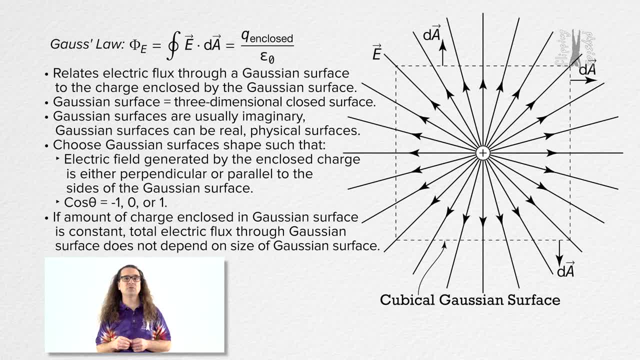 Correct, Billy. And as long as the amount of charge enclosed in a Gaussian surface is constant, the total electric flux through the Gaussian surface does not depend on the size of the Gaussian surface. Again, we showed this with the example we just did. I will also point out that 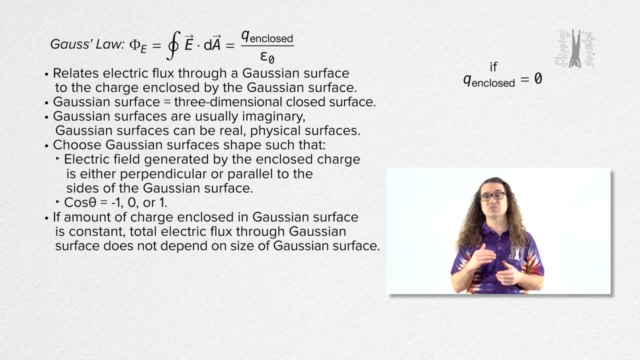 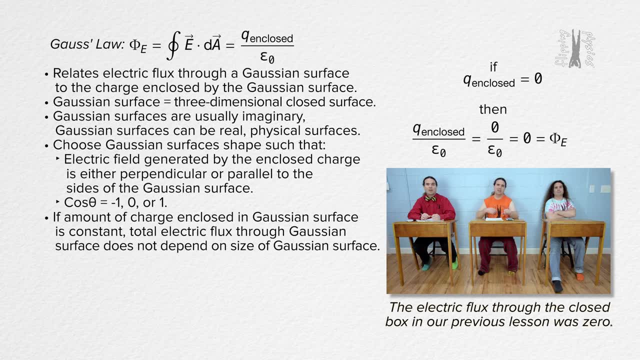 if the net charge inside a closed Gaussian surface is zero, then the net electric flux through the Gaussian surface is also zero. Oh, that is why the net electric flux through the right triangular box was zero. That is why you drank your tea. Thanks, Bobby, And thank you for learning with me today. I enjoy learning with you.